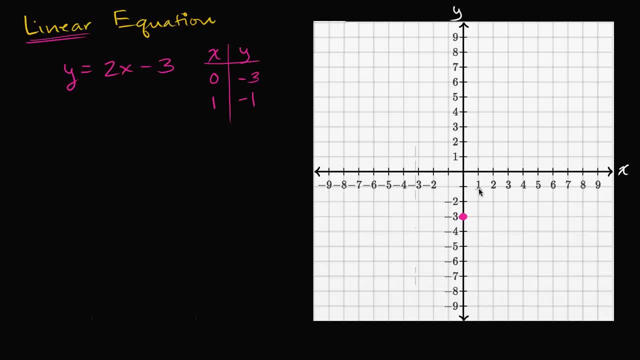 So we move positive one in the x direction and negative one or down one in the y direction. Now let's see: if x is equal to two, what is y? Two times two is four minus three is one. When x is equal to two, y is equal to one. 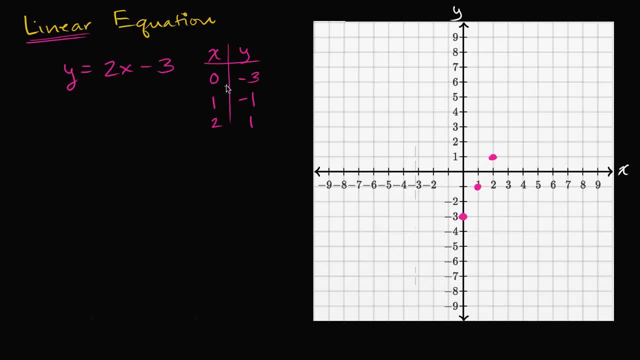 And hopefully you're seeing now that if I were to keep going- and I encourage you to, if you want, pause the video- try: x equals three or x equals negative one, and keep going. you will see that this is going to generate a line. 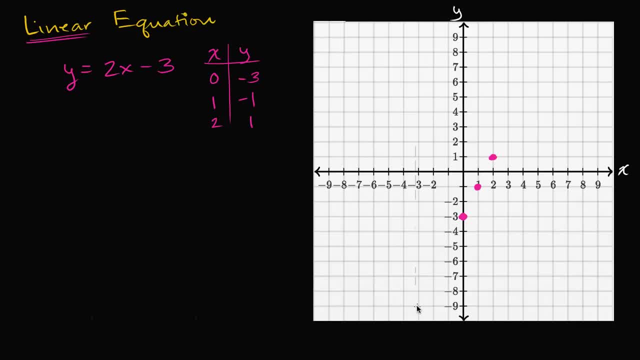 And in fact, let me connect these dots and you will see the line that I'm talking about. So let me see if I can draw. I'm gonna use the line tool here. I'll try to connect the dots as neatly as I can. 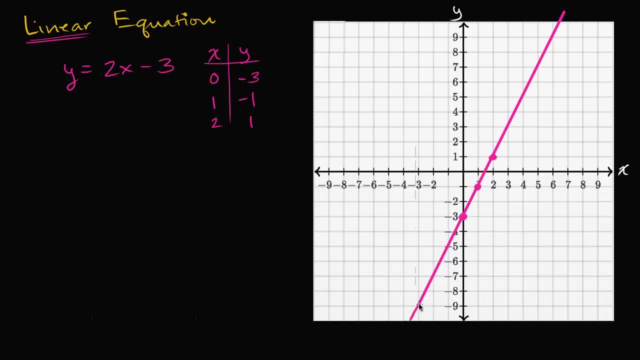 There you go. This line that I have just drawn- this is the graph. this is the graph of y- is equal to two x minus three. So if you were to graph all of the x- y pairs that satisfy this equation, you are going to get this line. 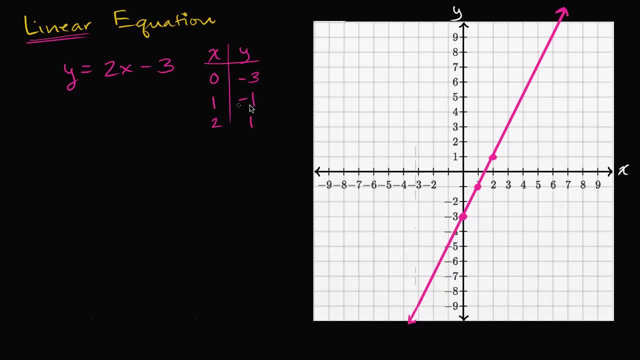 And you might be saying, hey, wait, wait, hold on, Sal, You just tried some particular points. Why don't I just get a bunch of points? How do I actually get a line? Well, I just tried over here. 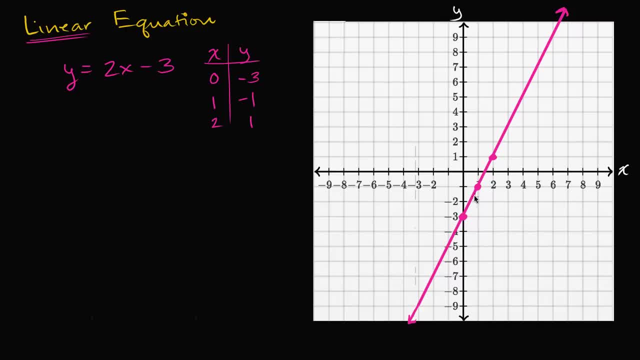 I just tried integer values of x, but you could try any value in between here, All of these. it's actually a pretty neat concept. Any value of x that you input into this, you find the corresponding value for y. it will sit on this line. 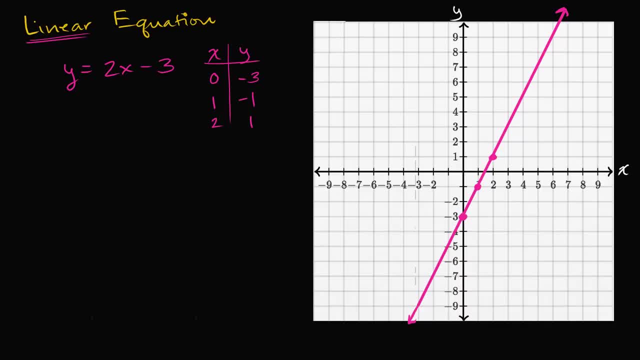 So, for example, for example, if we were to take x is equal to, actually, let's say x is equal to negative .5.. So if x is equal to negative .5,, if we look at the line when x is equal to negative .5,, 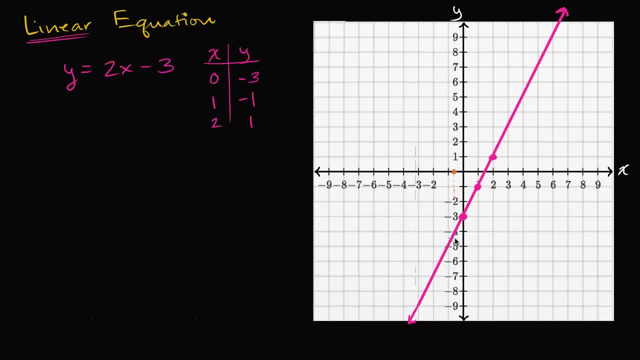 it looks like. it looks like y is equal to negative four. That looks like that sits on the line. Well, let's verify that. If x is equal to negative, well I'll write that as negative 1 1⁄2,. 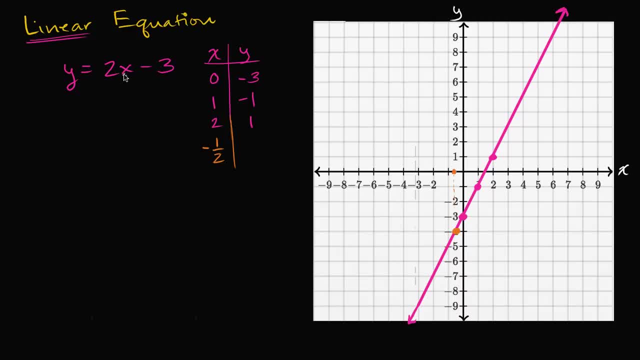 then what is y equal to? Let's see two times negative 1 1⁄2,. I'll try it out: two times negative, two times negative: 1 1⁄2 minus three. Well, this is two times negative. 1 1⁄2 is negative one. 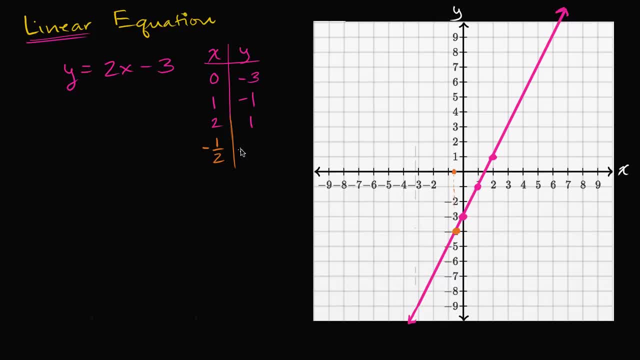 minus three is indeed negative four. it is indeed negative four. So you can literally take any, any for any x value that you put here and the corresponding y value. it is going to sit on the line. This point right over here represents: 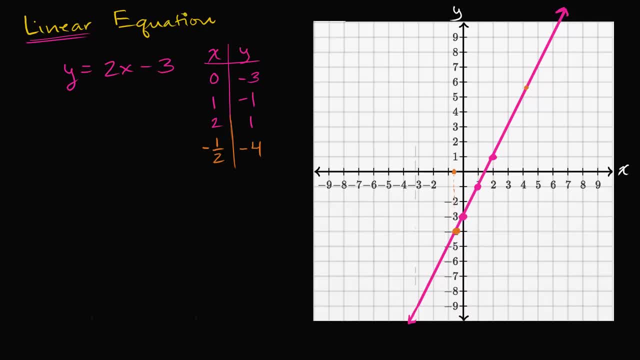 a solution to this linear equation. Let me do this in a color you can see. So this point represents a solution to a linear equation. This point represents a solution to a linear equation. This point is not a solution to the linear equation. So, if x is equal to five, 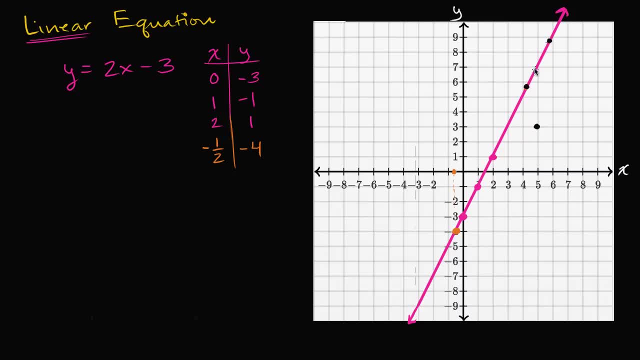 then y is not going to be equal to five, It's equal to three. If x is going to be equal to five, you go to the line to see what the solution to the linear equation is. If x is five, this shows us that y is going to be seven. 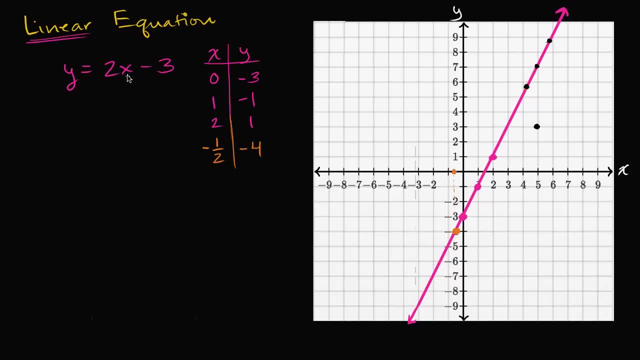 And it's indeed. that's indeed the case. Two times five is 10 minus three is seven. The point, the point five comma seven, is on, or it satisfies this linear equation. So if you take all of the xy pairs, that satisfy it. 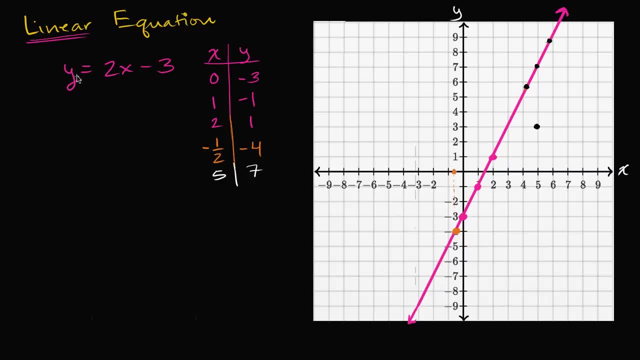 you get a line. That is why it's called a linear equation. Now, this isn't the only way that we could write a linear equation. You could write a linear equation like: let me do this in a new color. You could write a linear equation like this: 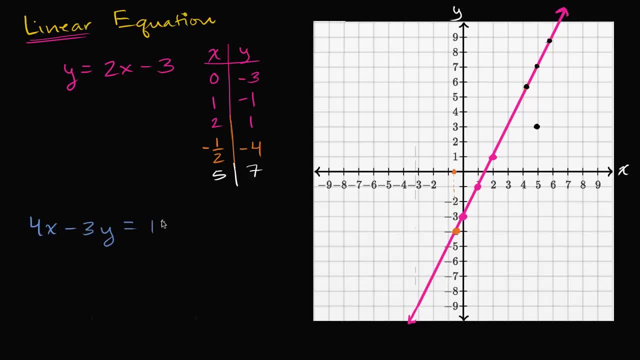 Four x minus three, y is equal to 12.. This also is a linear equation, And we can see that if we were to graph the xy pairs that satisfy this, we would once again get a line X and y. If x is equal to zero, then this goes away. 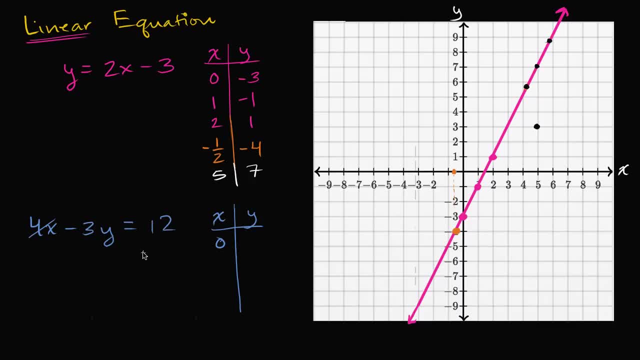 and you have negative three, y is equal to 12.. Let's see: if negative three y equals 12, then y would be equal to negative four. Zero comma, negative four. You can verify that Four times zero minus three times negative four. 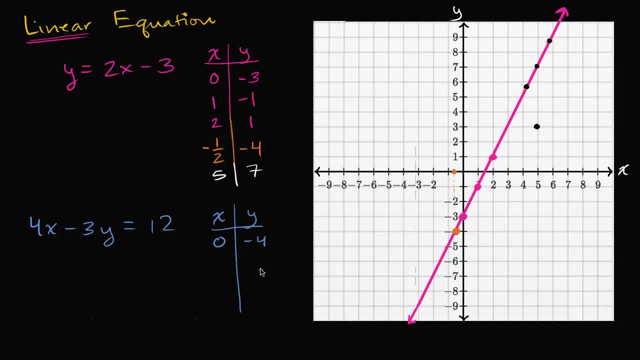 well, that's going to be equal to positive 12.. And let's see if y were to equal zero. if y were to equal zero, then this is going to be four times x is equal to 12.. Well then, x is equal to three. 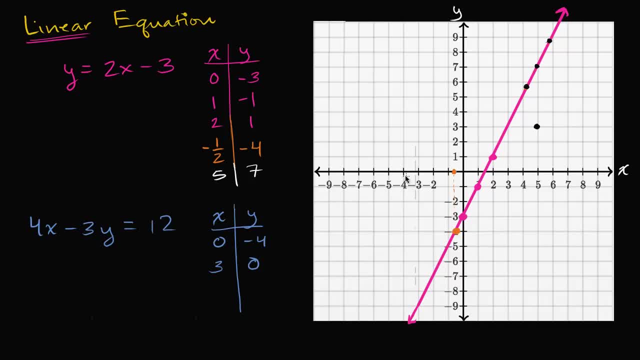 And so you have the point zero comma negative four. Zero comma negative four Negative four on this line, And you have the point three comma zero on this line. Three comma zero. Did I do that right? Yep, So zero comma negative four. 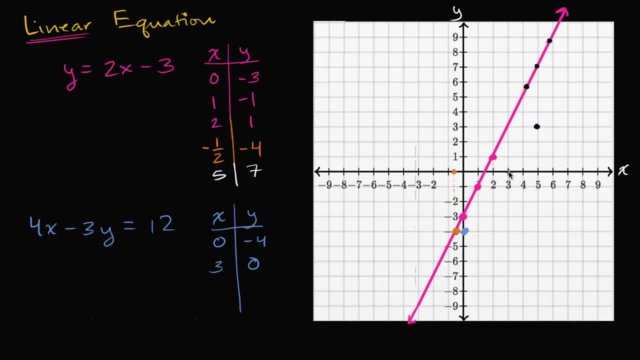 And then three comma zero. These are both going to be on this line. Three comma zero is also on this line. So this line is going to look something like- something like I'll just try to hand draw it- Something like that. 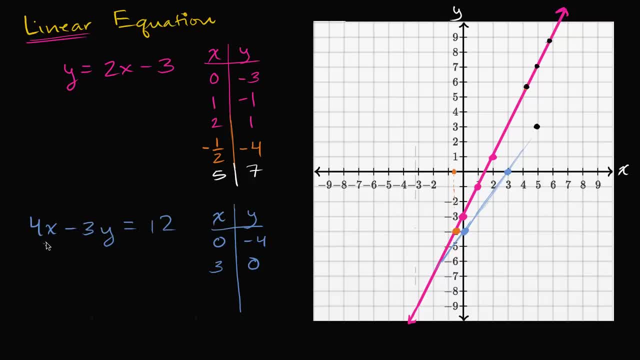 So, once again, all of the xy pairs that satisfy this. if you were to plot them out, it forms a line. Now, what are some examples of? maybe you're saying, well, isn't any equation a linear equation? And the simple answer is no. 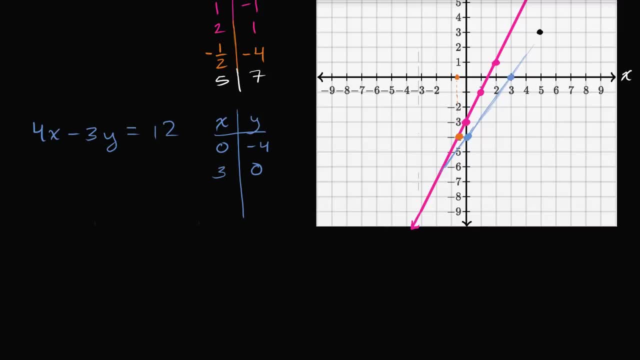 Not any equation is a linear equation. I'll give you some examples of non-linear equations. So a non non-linear- whoops Need to write it a little bit neater than that. Non-linear equations: Well, those could include something like: 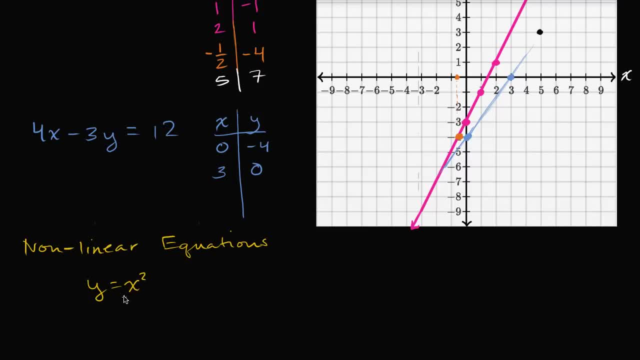 y is equal to x squared. If you graph this, you will see that this is going to be a curve. It could be something like x times y is equal to 12.. This is also not going to be a line, Or it could be something like five over x. 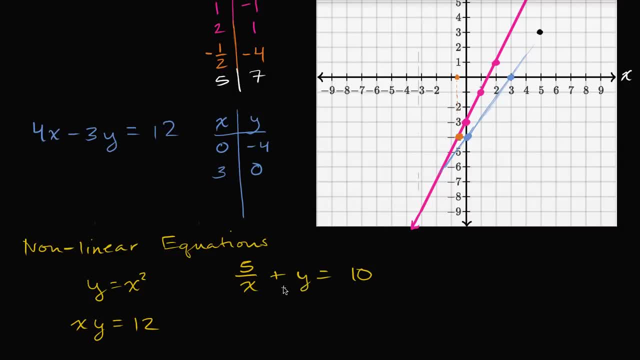 plus y is equal to 10.. This also is not going to be a line, So now and at some point you could, I encourage you to try to graph these things. These are actually quite interesting, But given that we've now seen examples, 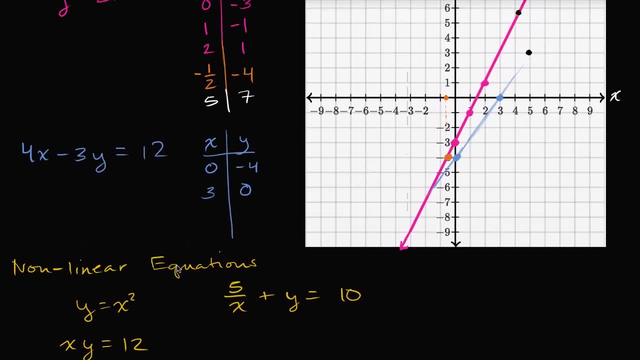 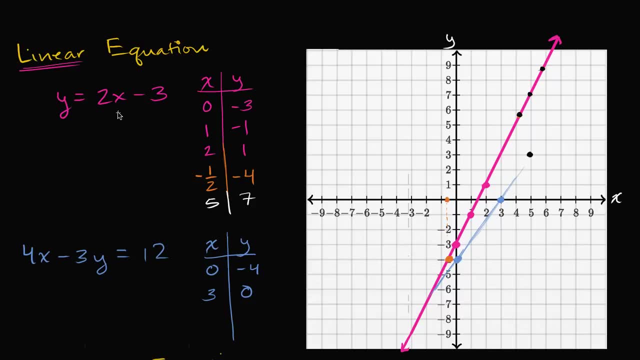 of linear equations and non-linear equations. let's see if we can come up with a definition for linear equations. One way to think about it is: it's an equation that if you were to graph all the x and y pairs that satisfy this equation, you'll get a line. 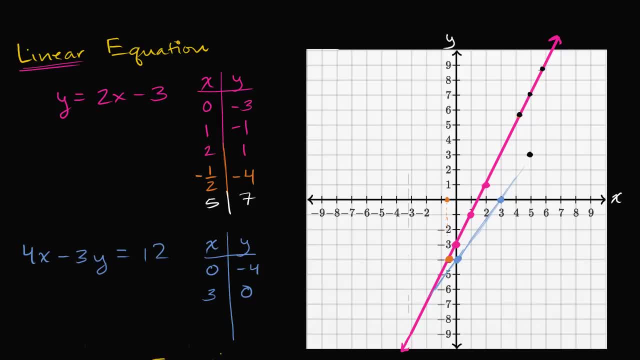 And that's actually literally where the word linear equation comes from. But another way to think about it is: it's going to be an equation where every term is either going to be a constant- So, for example, 12 is a constant. It's not going to change- based on the value. 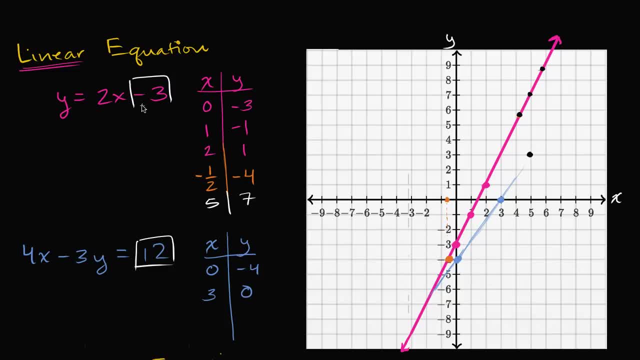 of some variable. 12 is 12. Or negative 3 is negative 3.. So every term is either going to be a constant or it's going to be a constant times a variable raised to the first power. So this is a constant two times x to the first power. 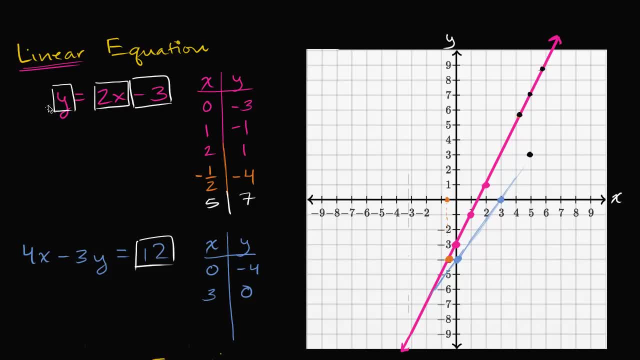 This is the variable y raised to the first power. You could say this is just one y. We're not dividing by x or y, We're not multiplying, or we don't have a term that has x to the second power or x to the third power.